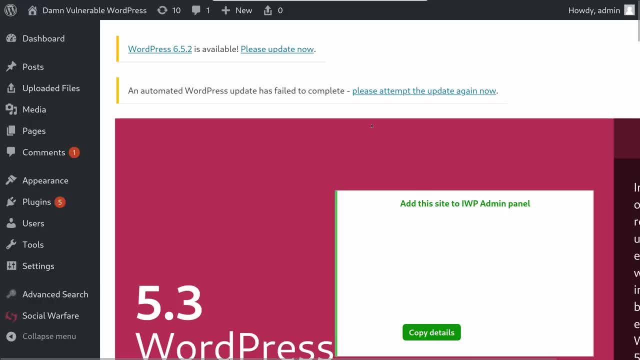 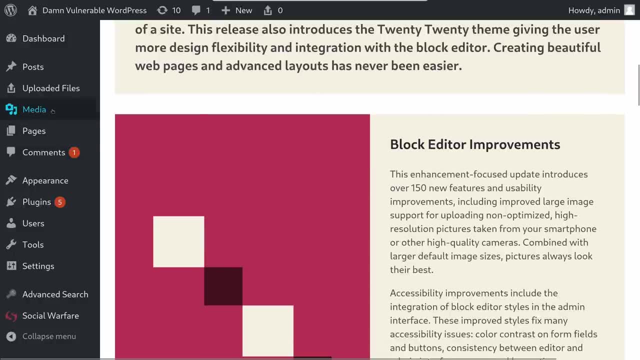 Today, I'll be teaching you how to hack WordPress. WordPress is a content management system that allows you to very quickly be able to set up a website across the internet and have your different modules, pages, posts that you can create across the internet. Basically, it's a system that allows: 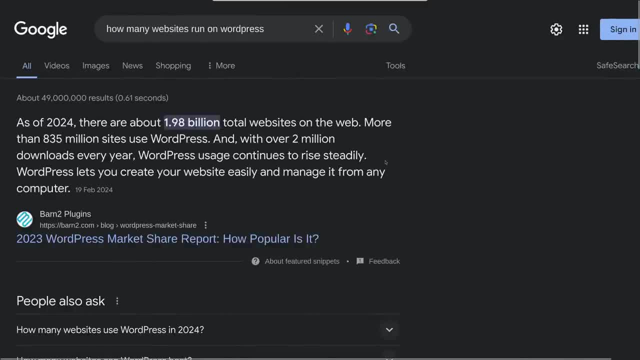 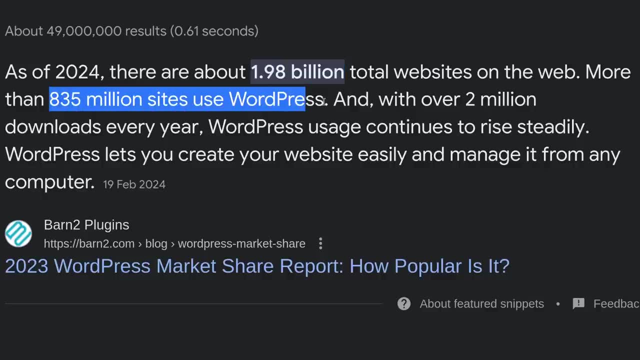 you to host websites, And if you do a quick search on how many websites run on WordPress, you can see right here: there are 1.98 billion total websites on the web. More than 835 million of these sites use WordPress. So, yes, I'll teach you how to do penetration testing on WordPress. 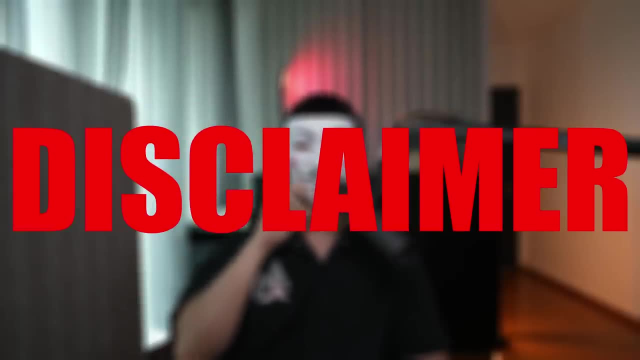 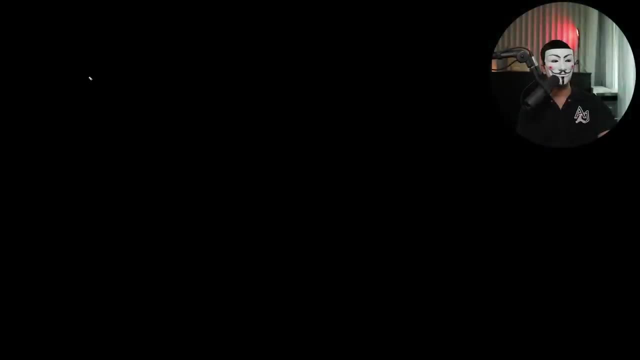 sites. Now, before we get started kids, remember hacking is illegal. If you want to hack, remember to ask your mom for permission first, And if you get caught hacking, do not tell them you know who is Mr Hackaloy. So, when it comes to the architecture of things, we first have a target website that 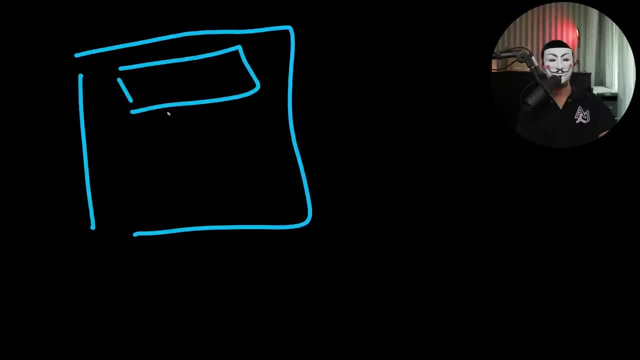 we're going after. So it could be internet facing or it could also be facing the internet, It doesn't matter. As long as it's running on WordPress, we are able to target it. Next up, we have your BFF, Mr Hackaloy, who can be targeting the site, running different type of hacking techniques. 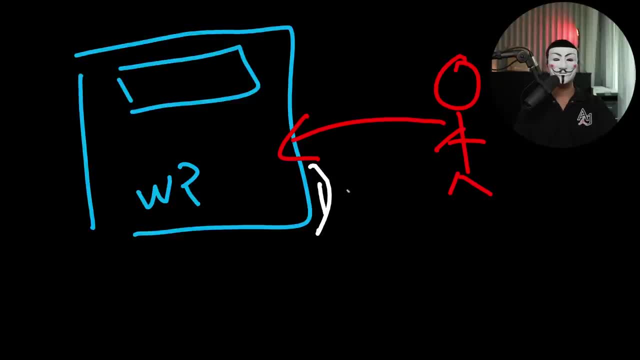 that are specific against the WordPress site One. typically, we want to enumerate different parts of the pages. For example, we could be looking for admin pages, we could be looking for wp-content, looking for plugins and so on- And once we have all of these details, what we can do now is to go ahead and search up the specific 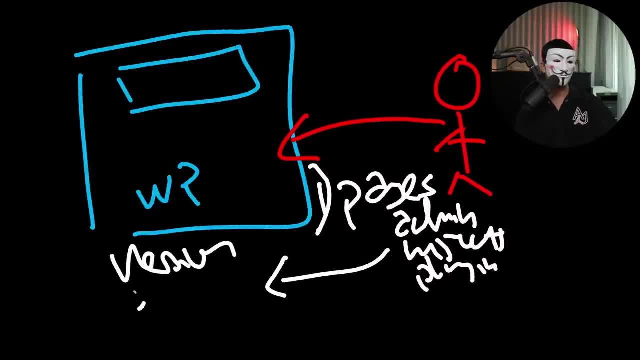 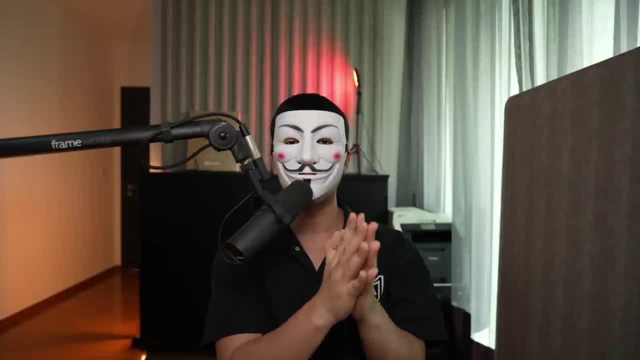 version of all of these different plugins, as well as WordPress itself, to look for exploits that we can use to directly target and break into the site. And for today's case, we'll be doing SQL injection attack, as well as the ability to take complete control of the entire site. 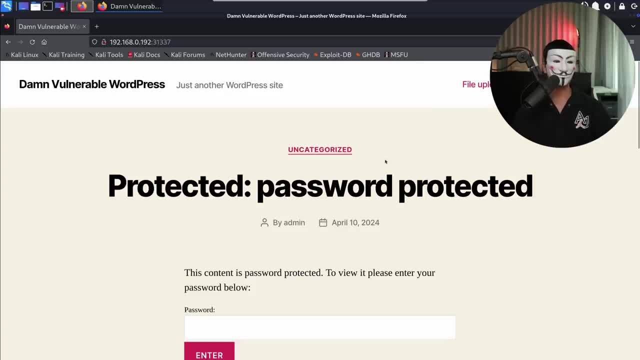 So let's go ahead and get started, So let's go ahead and get started, So let's go ahead and get started. So, right in front of us we have WordPress running. So this is a website. It could be a website from the. 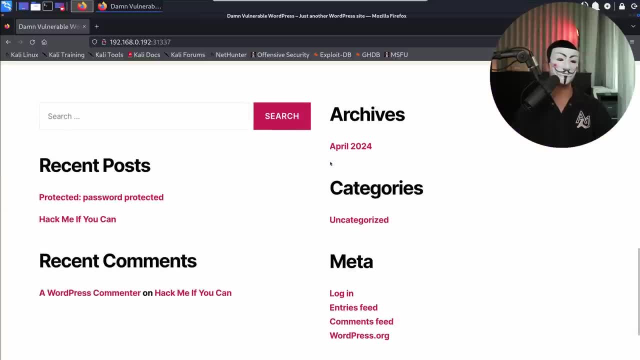 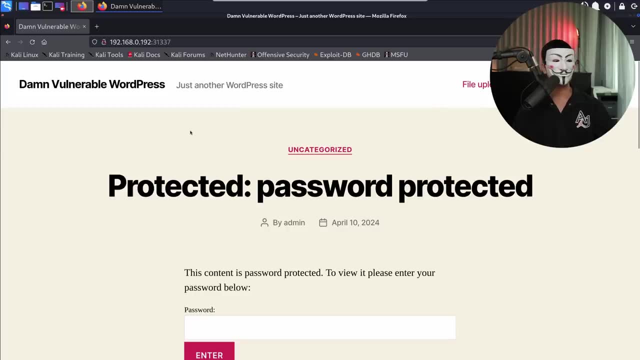 internet. It could be a website that you're hosting and you're testing it all, or it could be just another internal system that you could be targeting. So the first thing we want to do is to look for the WordPress version. So what you can do is you can go to the site. 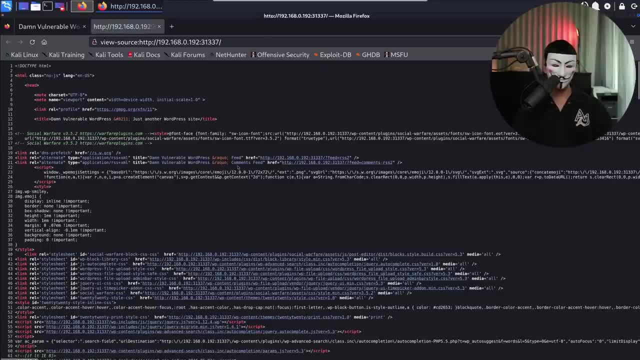 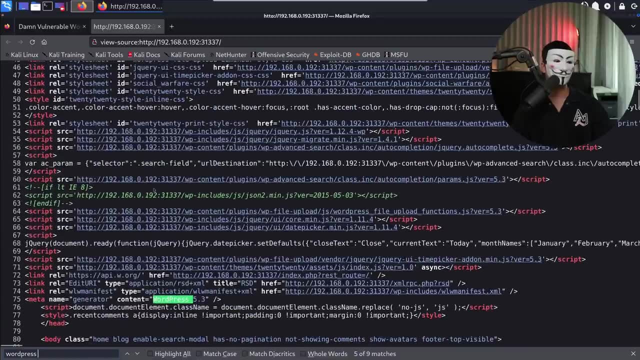 itself, do a right click and click on to view page source And from there you can go ahead and enter WordPress space and see if you could find a specific version of it. So in this case, if you zoom in a little more, you can see right here that we have a specific version. 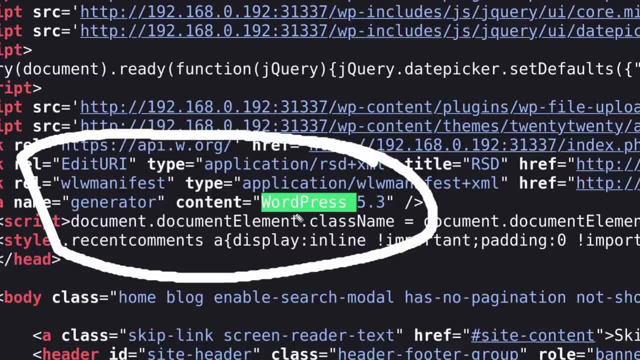 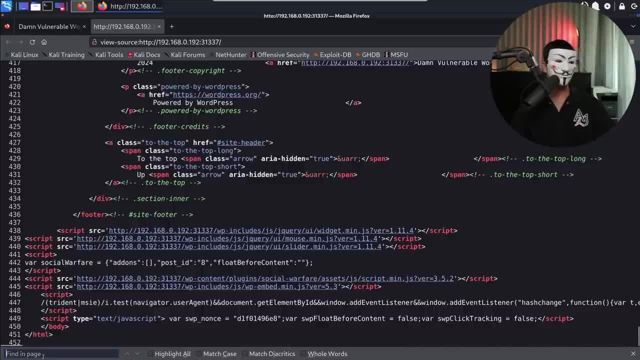 So in this case we have the following of WordPress 5.3.. The other two options also look for JavaScript as well as CSS file that could be indicating of its version. So what I can do now is go ahead and search in the page for js question mark version equal. 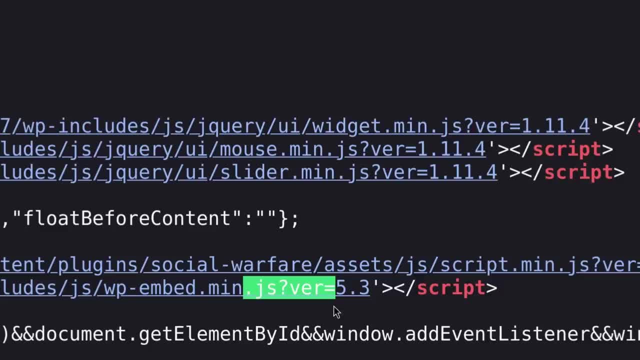 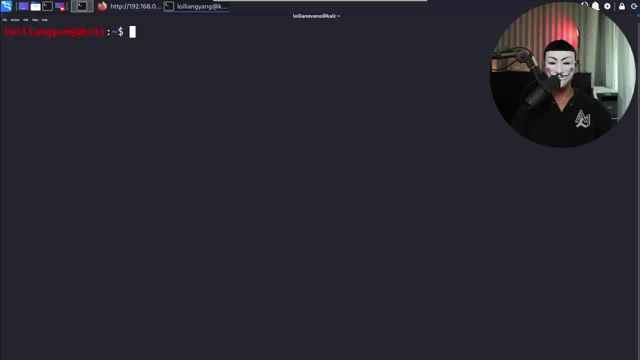 So in this case you can see right here we have the following of version 5.3. And the other one for CSS file. we can see: right here too, we have the CSS question mark, version equal 5.3. And with that we can go over into a service like SearchSploit to look for the 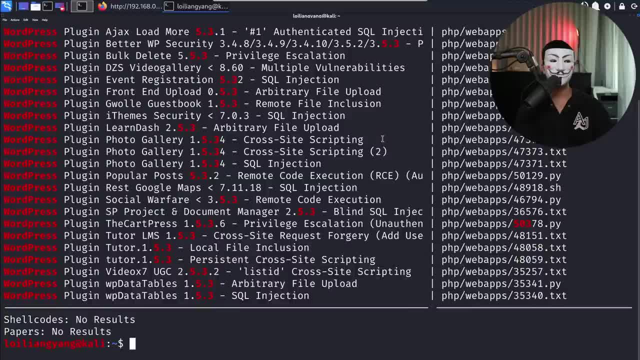 word, press 5.3 and see what we get as a result from it. So SearchSploit is a way for us to look for those available exploits that we could use as part of targeting the site. So in this case you can see the following of WordPress. So typically we're seeing plugin. 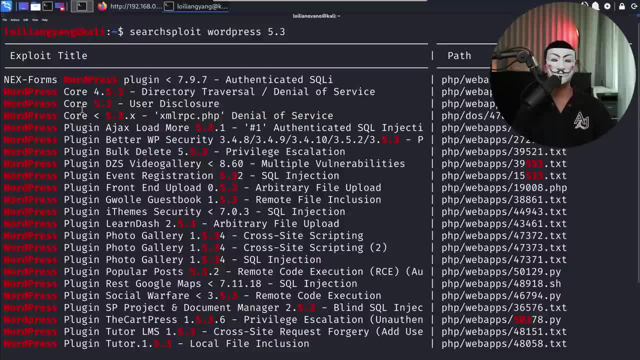 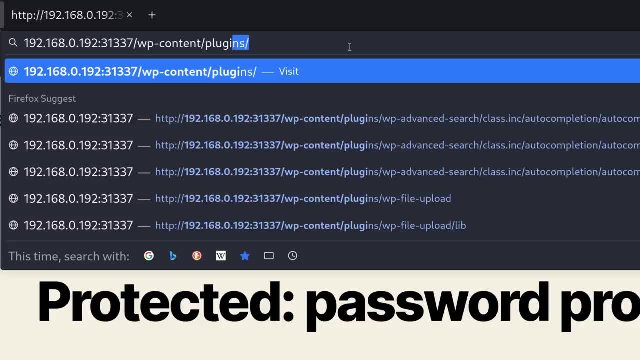 we could also see core user disclosure and all this different information that we can quickly use as part of targeting the site, because it's been unpatched. The other page is really big- is wp slash plugins. Hit enter on this And right now you do not see any. 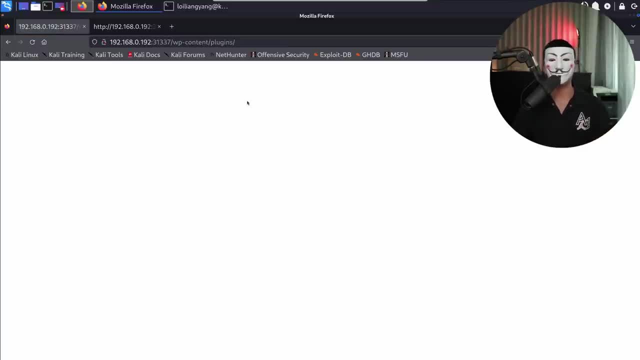 listing of what's in the list. So look for this And look for WordPress 5.3. And this- those plugins- is available against the site. however, what we can do now is to use a trick to test whether the plugin exists by entering the plugin itself into the uri, for example, over here. 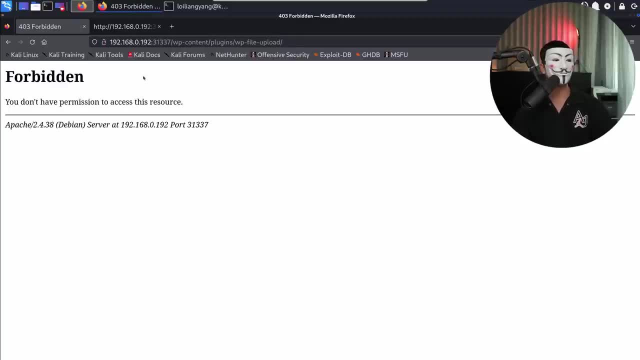 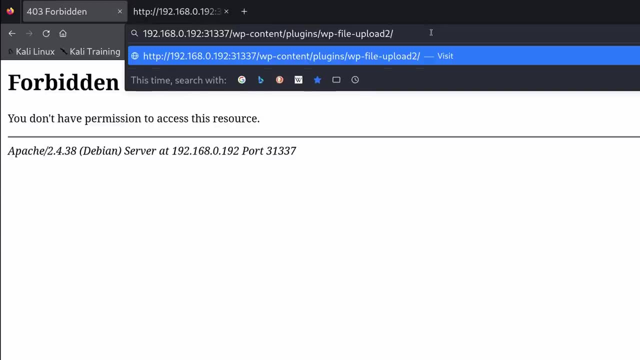 i have wp file upload. i clicked on it and you can see right here it states forbidden. you don't have permission to access this resource. however, if i was to go ahead and enter wp-file-upload2, which is not a plugin, i hit enter on that. it stays the following: the requested url was not. 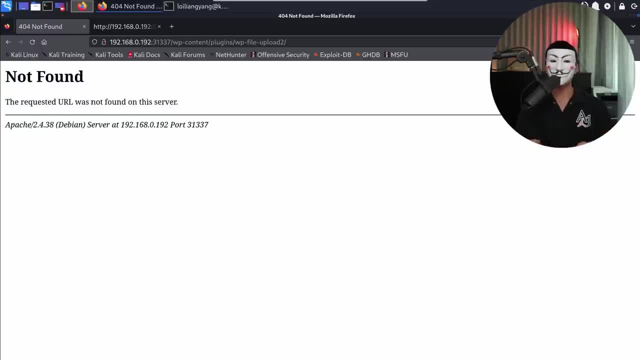 file on this server. so what does it mean? it means that there isn't such a plugin installed. the other example is here as well. in the wp advanced search. i hit enter on this. so once again it says the following: forbidden: you don't have permission to access this resource. however, if i want to change, 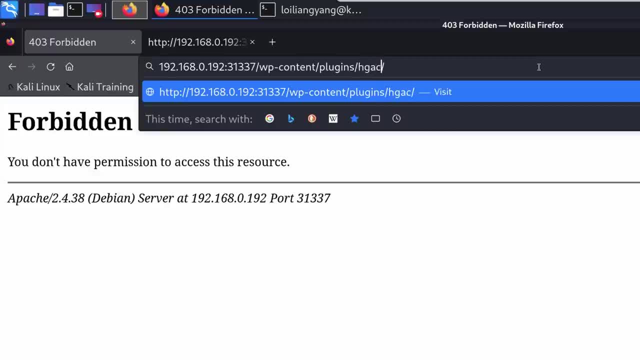 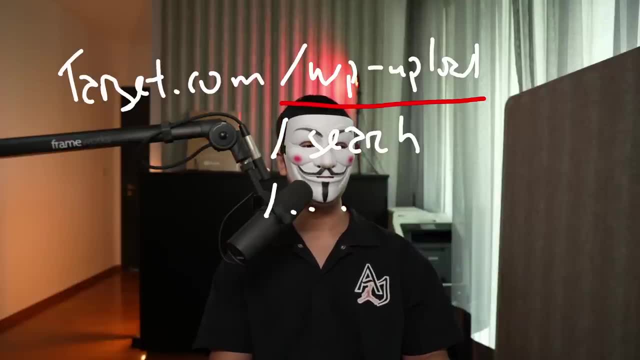 it up to some other plugin name, so say, for example, hacker alloy plugin. i hit enter on that, not found. there isn't such a url. so what we can do now is start targeting all these different common plugins, as well as pages, so that we can identify the structure of the site. so what i can do here is: 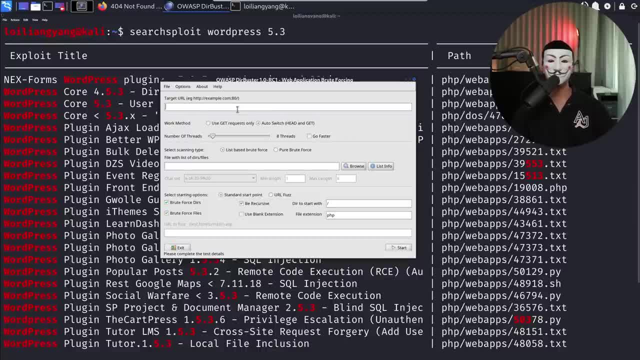 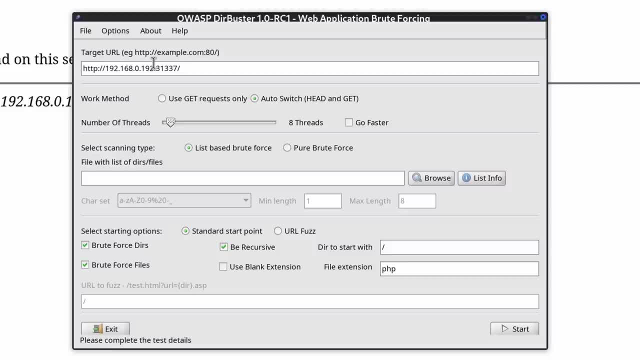 use a tool like this, ir buster, to be able to help us target the site. all you got to do is go back over into the site, copy the url, copy on that, paste it over here and we have the number of threads and all this information. what's most important is the file with list of directories of files. so go ahead. 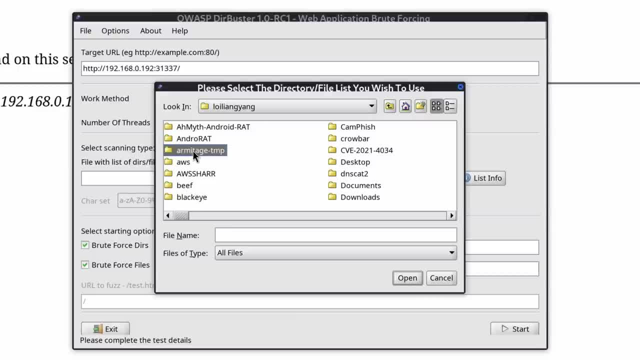 and click browse and with that we can go over into usr. let's head back over into root, into usr share, followed by word list, hit enter on that and we have dir, buster, buster, clicked on that and we can use something like a directory list, small. so all this are. 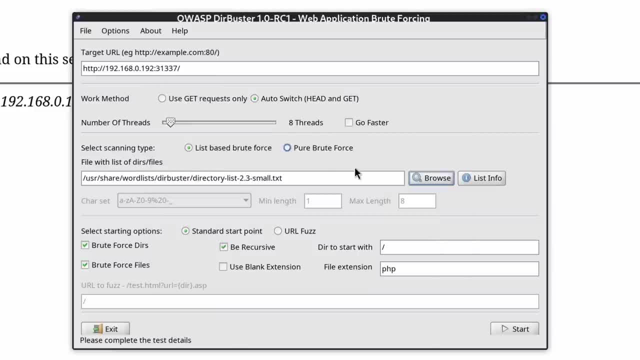 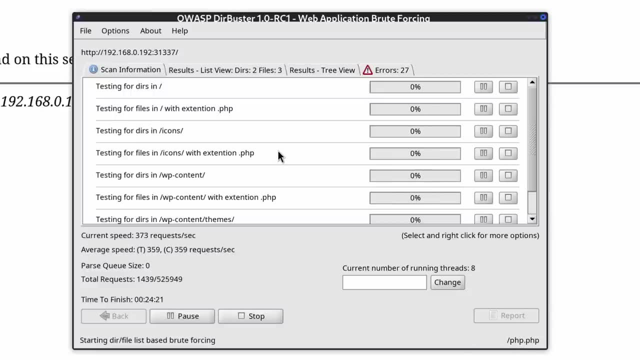 already available out of the box with column linux. double clicked on that and we can go ahead and click start and we'll be trying to find out all these different parts of the site that has all these pages, plugins and so on, and as we're running the attack, you can see the list view directories. 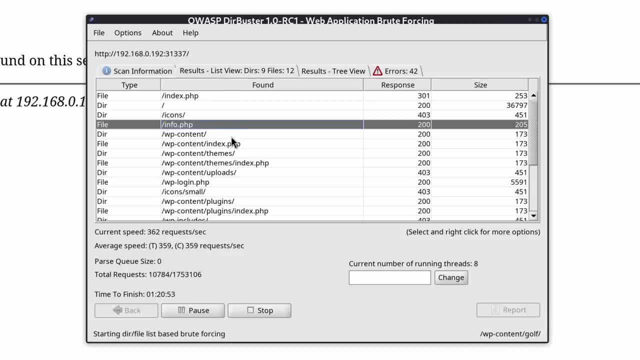 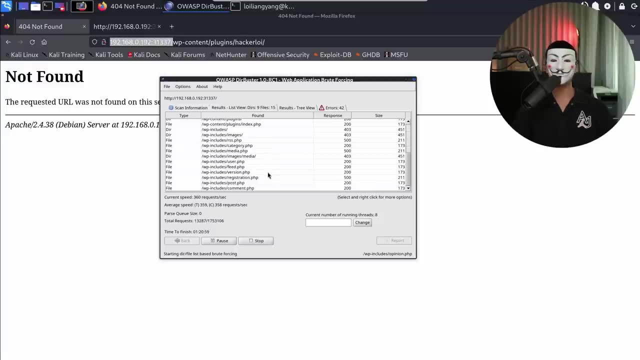 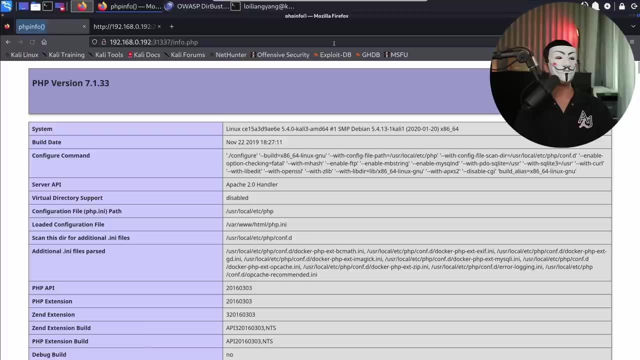 we have infophp, which is very juicy information with wp-contentindexphp, teams uploads, wp login and so on. so all this, all these things, are already available out of the box with column linux. double click on that and we can go ahead and hit enter and that and boom. this gives us incredibly. 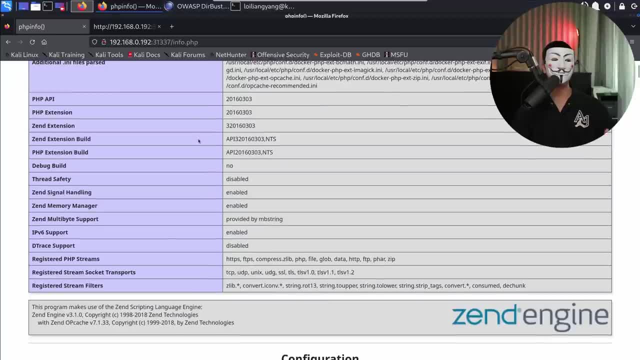 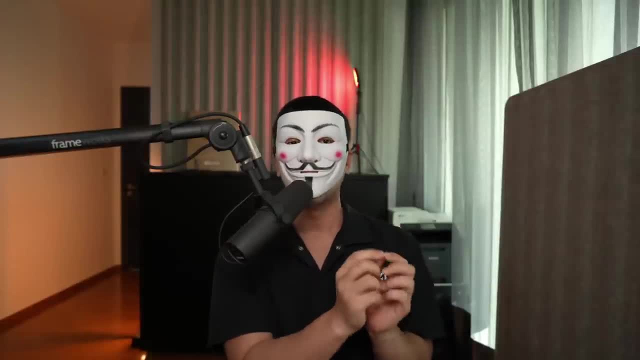 important information, like the php version, and as we scroll down further, we can see all these different details that can help us target the site more tightly. now the even better part is we have specific tools that we can use to target wordpress site, and it's called the wp scan, and 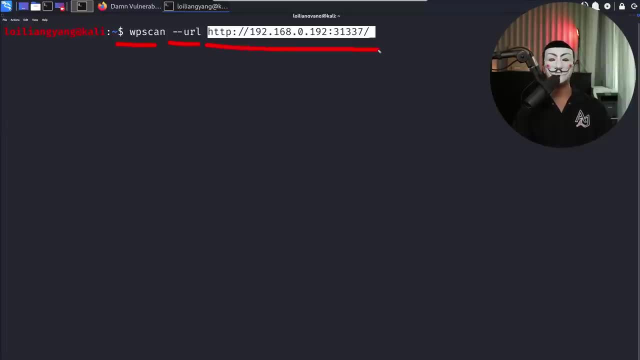 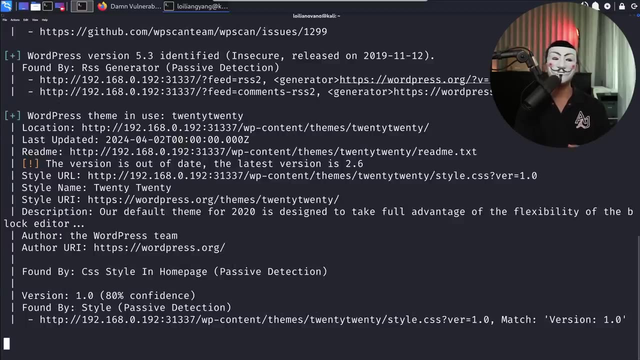 all i'm going to do is enter the wp scan dash, dash url, followed by the target site, and that's all. and once you're ready, go ahead and hit enter on that. i will begin scanning the site, looking up for all this different information that we were trying to do earlier, but more specifically targeted. 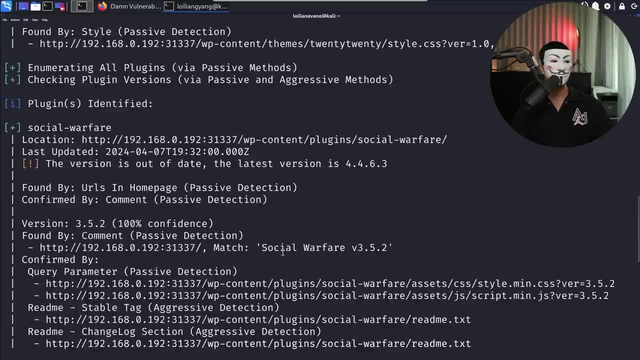 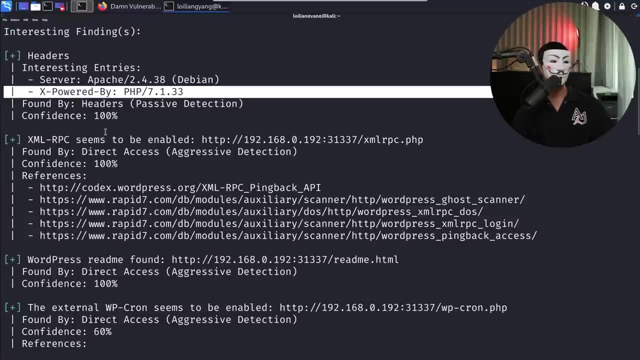 towards wordpress and we got really good information. so if i scroll all the way back to the top trying to understand the findings, so we have interesting findings here. so we have the server apache php. we have xml rpc that's enabled, that we can target. we have the wordpress readme file. 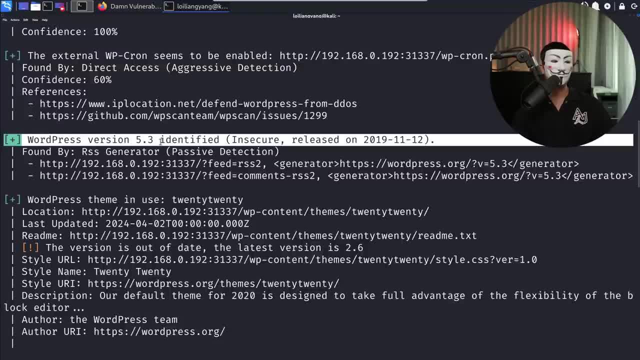 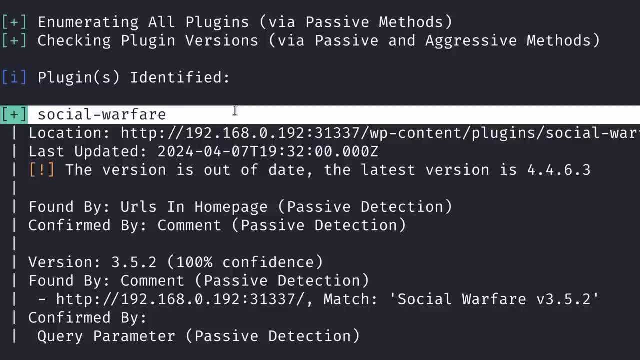 we have the w chrome and so on. so all this are the different things that we can do here. so we can view the original user file, for example. we can do this here, so let's do that. here we can see that we have a different identification of the version. 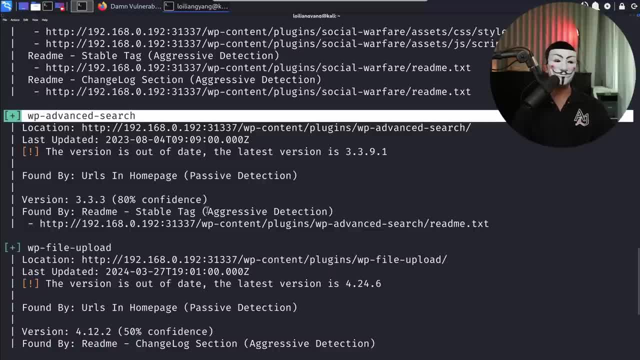 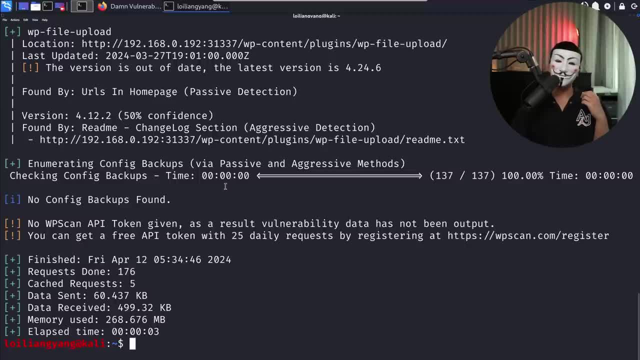 different identification of possibly plugins on the site, like, for example, for example, with social warfare. we have the wp advanced search and it's telling us that the version is out of date and we can target them directly. however, there's something even better is that we can automatically use the. 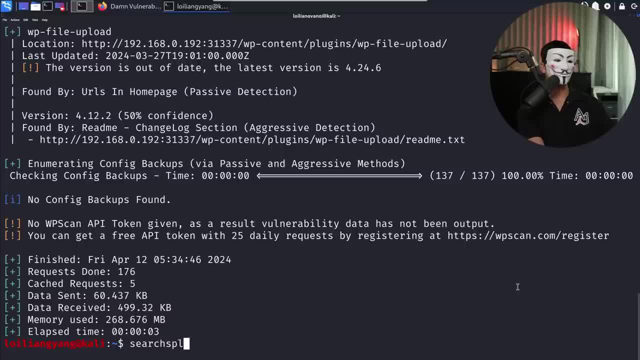 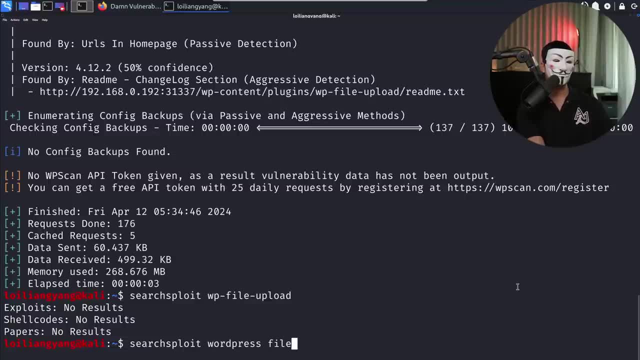 wp scan api token that can help us match all this plugin versions to available exploits that we can file dash upload. i'll hit enter on this now. results are in to say wp: wordpress file upload. all right, trying to find for specific versions and so on. so you can see here that i've already. 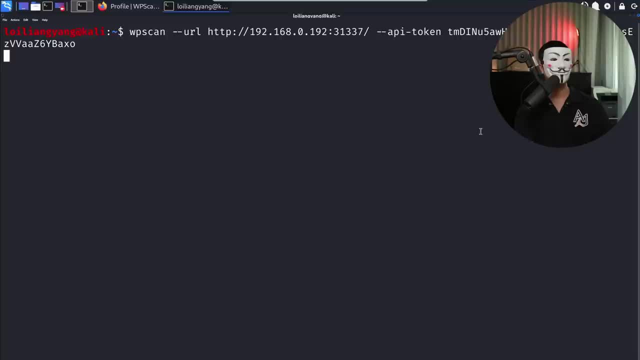 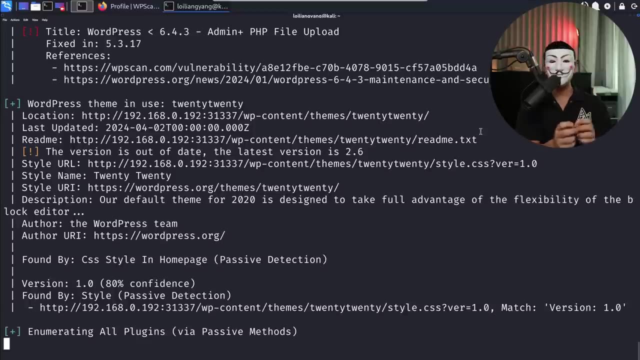 taken my api token. i'm ready to hit the site, so go ahead and hit enter on this, and now we're scanning. we're doing the same scan. however, we are saving precious time now by having the matching against those exploit database automatically for those plugin versions, for any other things. 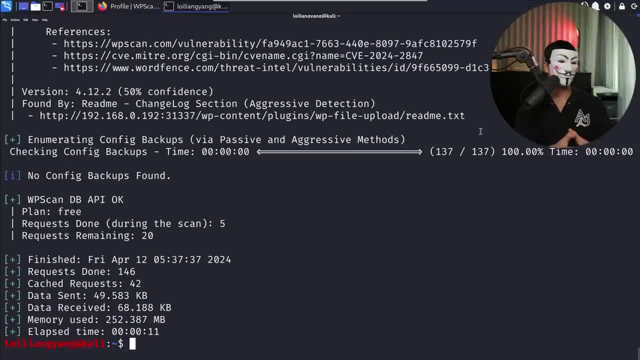 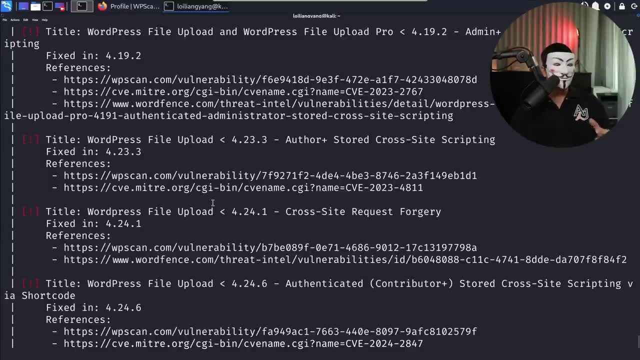 on the wordpress site: boom done, the scan completed and we can scroll all the way back up again. and as we're scrolling up, we can see all this different information, like wordpress file upload, author plus start, cross-site scripting and so on. so this helps us narrow down on the specific. 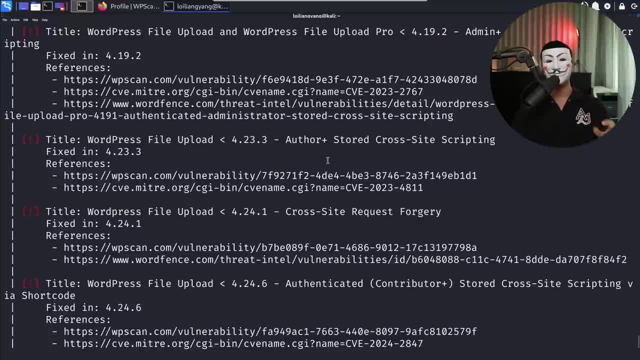 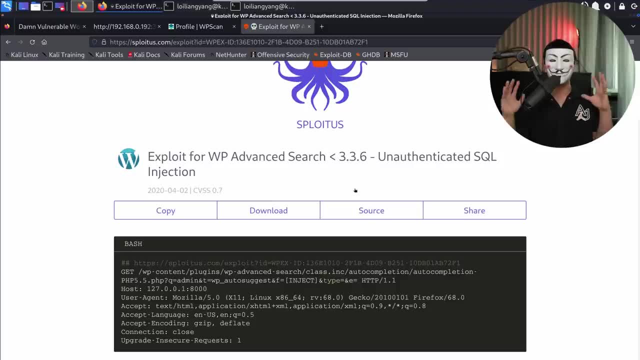 exploits that we can use so we can send those malicious payload against the target site. and for today, i'll be teaching you wp advanced search- unauthenticated sql injection attack. and we are exploiting the wp advanced search- unauthenticated sql injection attack. and we are exploiting the wp advanced search- unauthenticated sql injection attack. and we are exploiting the wp advanced search. 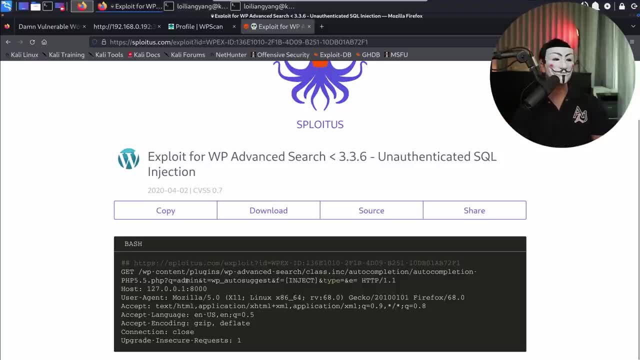 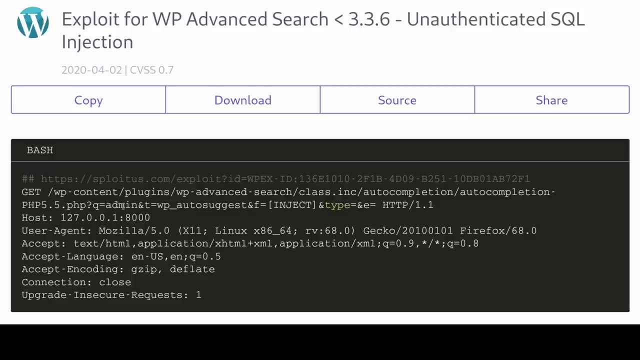 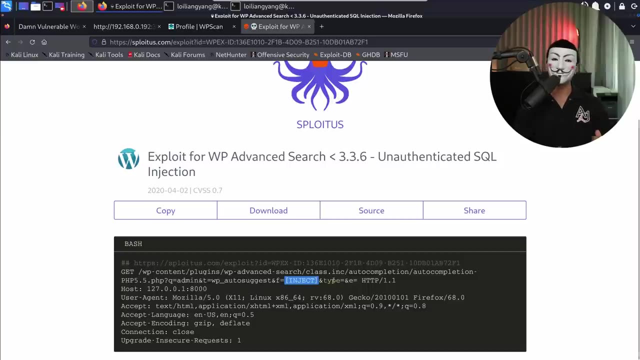 right here and we have the exploit for wp advanced search and we can see right here we have get wp content plugins and we're targeting a costinc auto completion and of course we have the following queue: equal admin, wp auto suggest and this is the injection point. so the great thing is, if you saw, 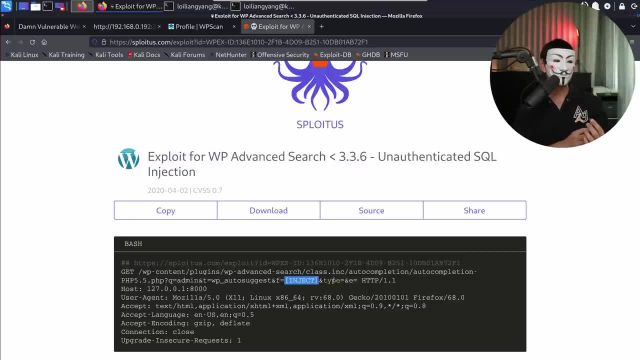 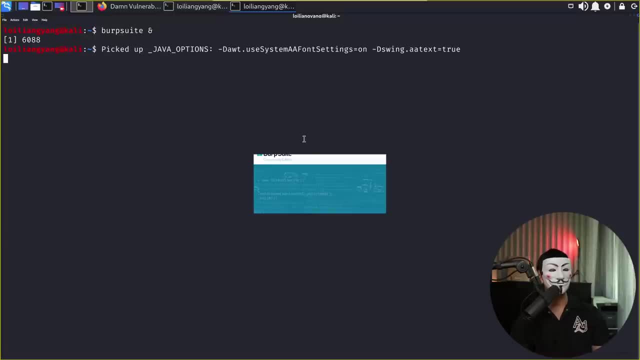 from the earlier tutorial, we could directly use sql injection attack to target this part of the site. so what i'll do right here is to go ahead and enter burp suite, open this up, launch it, and what i can see right here is where burp suite launching and we have the community edition go. 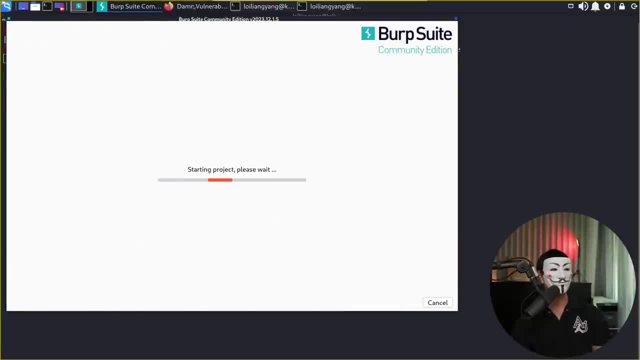 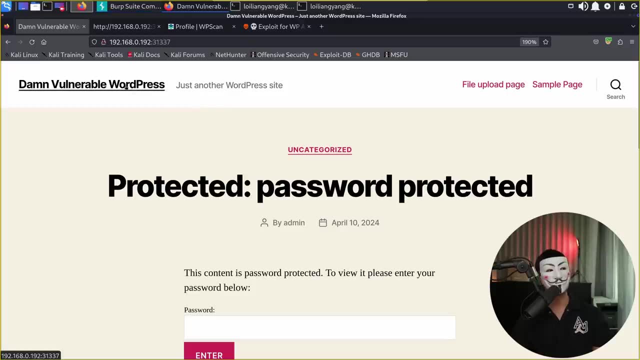 ahead and click next, click start burp and once we have that we'll be able to start the proxy and begin intercepting all of this request. so if i head back over here i'll just go ahead and click onto the site. we go on the proxy tab. we have an example of the request. i do a right click on this. 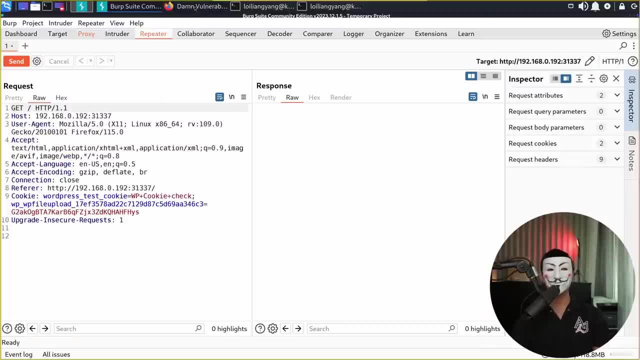 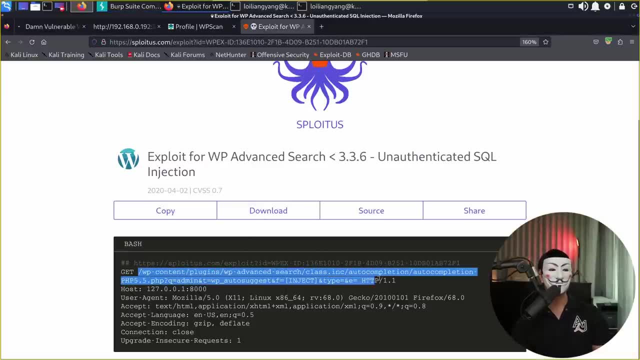 i send over the repeater and from repeater i have to change things up a little bit, so i head back over to exploit this, and what we want to do now is to change the request. so i'm going to go ahead and copy this to get your eye. so in this case, this is the one that we'll be using. i can go ahead and. 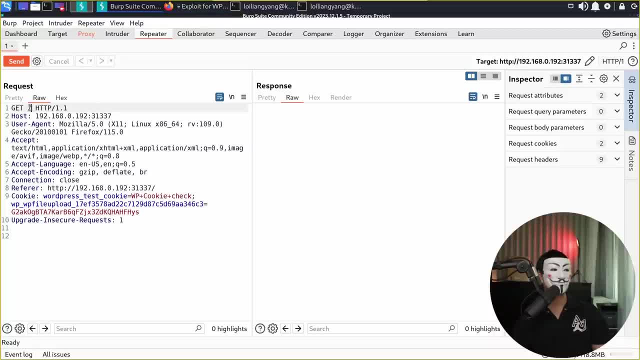 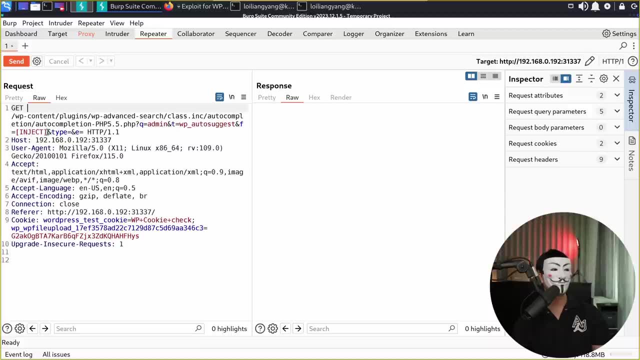 copy this head back over into burp suite or i'll go ahead and paste it over and you can see right here. this is the example of wp content and so on and so forth. and what i can do is i can change this over to star so the sql map, which is an automatic sql injection tool, can target this. 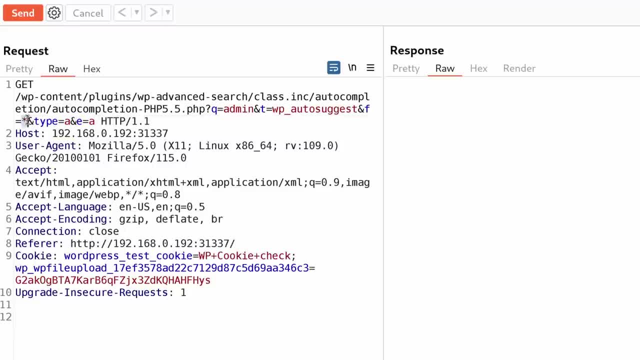 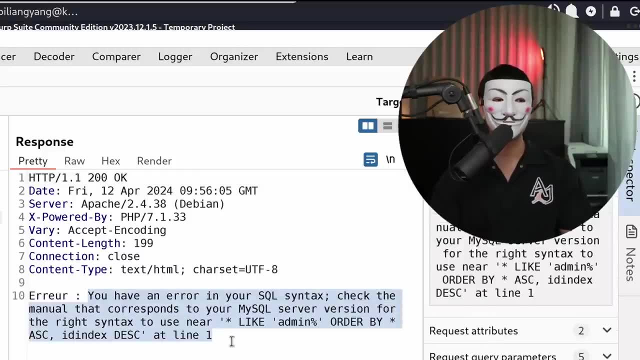 part of the site. in fact we can even test it right here so you can see the following of the site. i click send on this, it stays the following: you have an error in a sql syntax. check the manual. that corresponds to your my sql server and so on. so you can see right here. 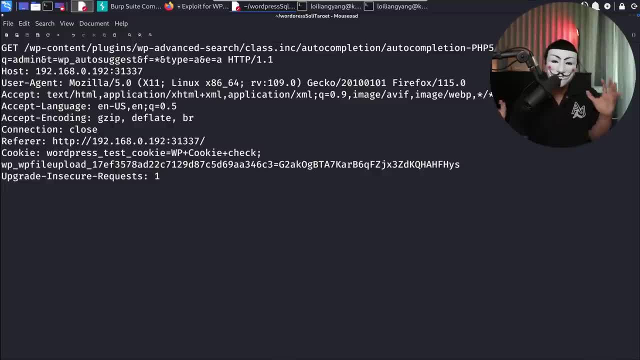 this is an example of a vulnerability. take it to the next level. i've saved this into a file that we can then use sql map, our automatic sql injection tool, to target the site, to automatically pull out those information from the site. you can see right here with sql map dash, our wordpress sql i target. 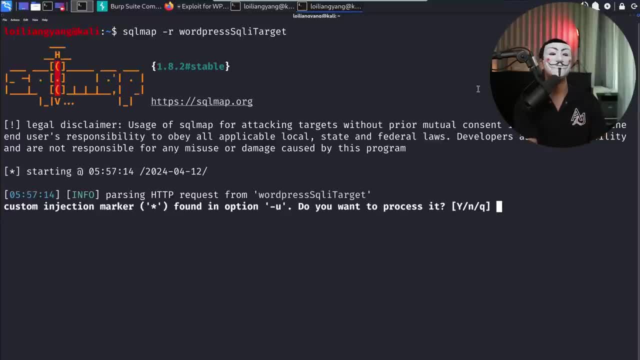 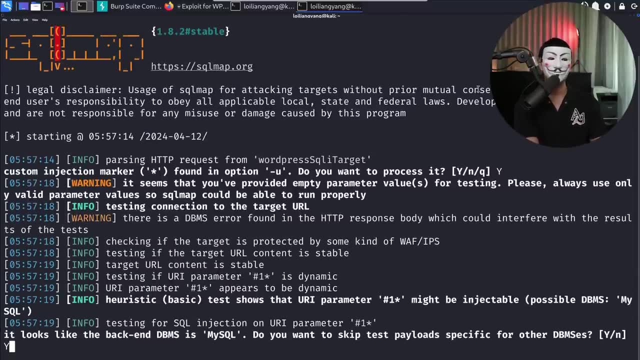 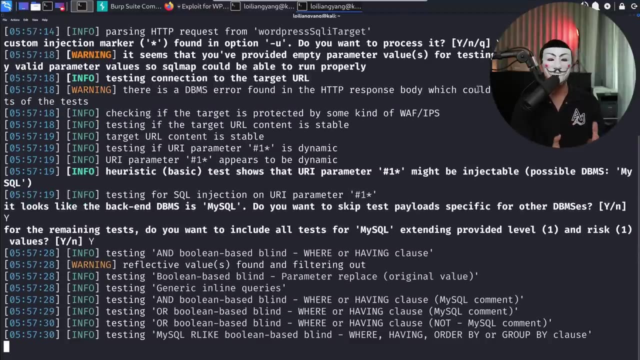 hit enter on this custom injection marker file. so we want to process it. and boom, it looks like the backend dbms is my sql. do you want to skip test payloads? yes for the remaining test. do you want to include all tasks enter? yes for that. and right now we are gaining access to the backend system. we are in. we've gotten through the 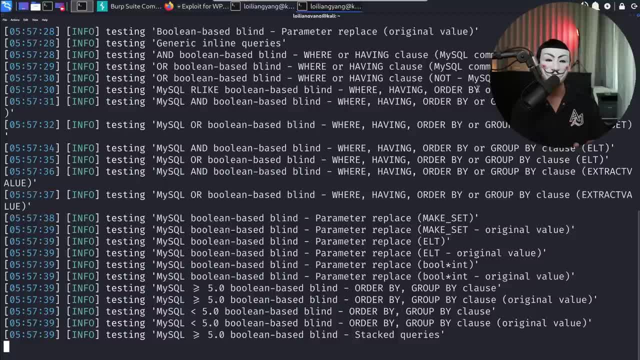 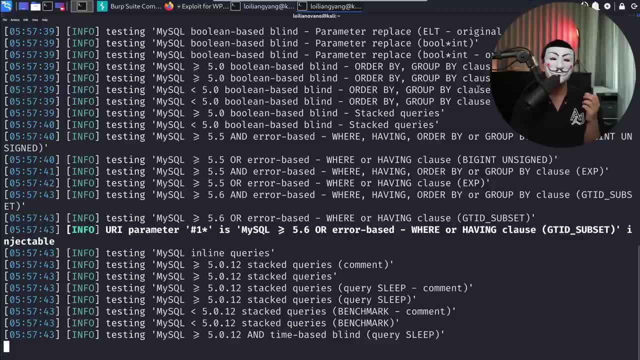 vulnerability of the sql injection attack. and right here we're scanning, we're running all these automatic queries and it makes dumping out the information, as well as the database, significantly more efficient and it makes it more efficient, and it makes it more efficient and it makes it significantly easier through this automation. 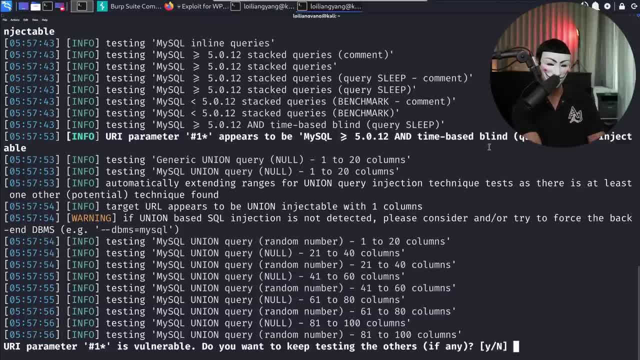 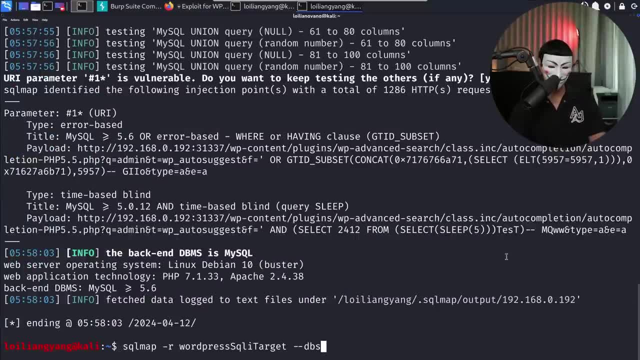 there you go. uri, premarital. one is vulnerable. do you want to keep testing the others? let's enter no for that. and right here we can go to the advanced query functions of sql map. now we can enter the following: of dash, dash dbs to look for all those available databases and the process. 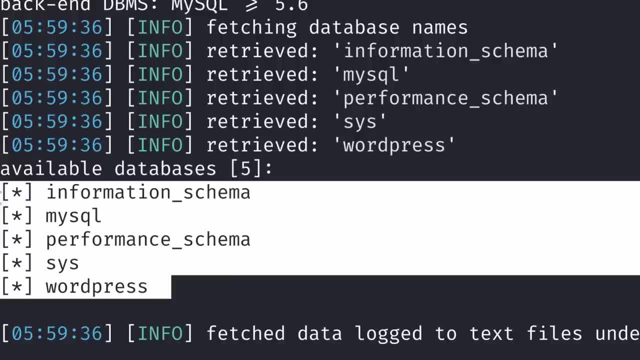 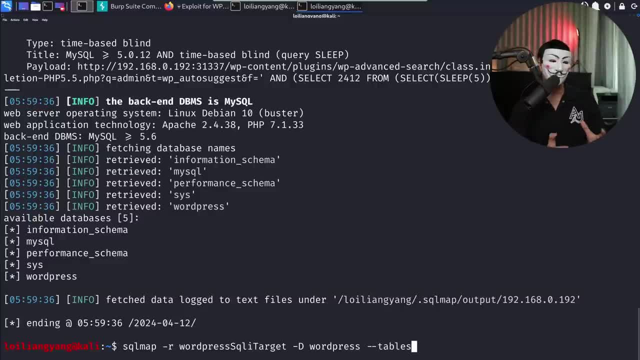 for it and you can see right here, and with the following of five databases: information schema- my- sql. and the following of five databases: information schema- mysql. and the following of five databases: performance schema- sys and wordpress. let's go ahead and target the wordpress database. now we'll switch things up a little. we're entering dash d to target the wordpress database and we 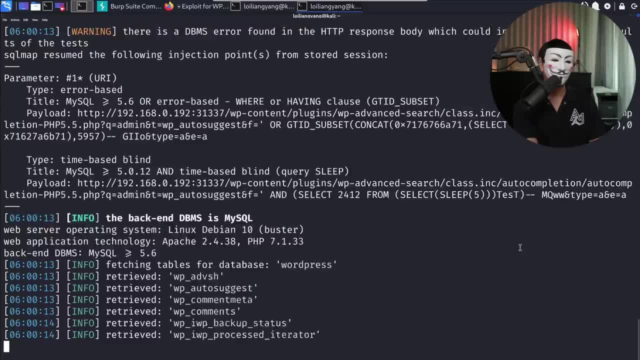 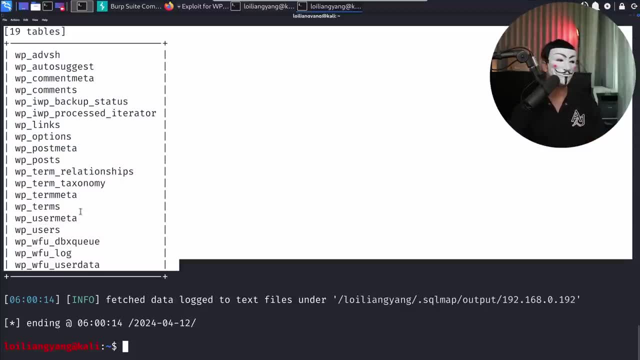 want to dump all of those tables. let's hit enter on that, enter yes and right here we can see that all these are the different tables that we can go after. we have 19 of those tables and let's go ahead and target the blue p underscore users and see what we get. so right here we are targeting the. blue p users table and we want to dump everything out here. do we need to do any debt window in our slash? this one is one of our big48, but we know how large the blind chart works. but we also want to do things like stretching spectrum millones. so we're going to select our area of a table that's going to get. 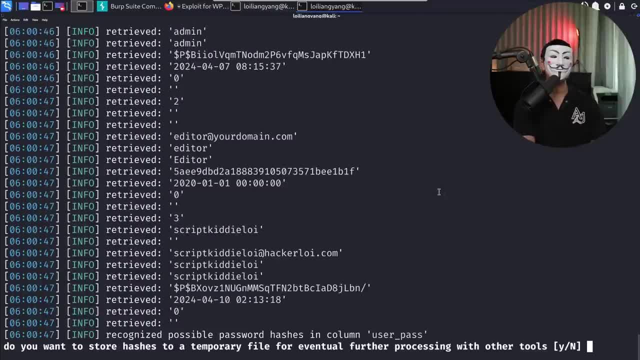 of the table: enter yes for that. now, right here, we are gathering all of those information. it even states the following: do you want to store hashes to temporary file for eventual processing? enter no for that. do you want to correct them via dictionary based attack? let's try it. hit enter on that. common suffixes: enter no. 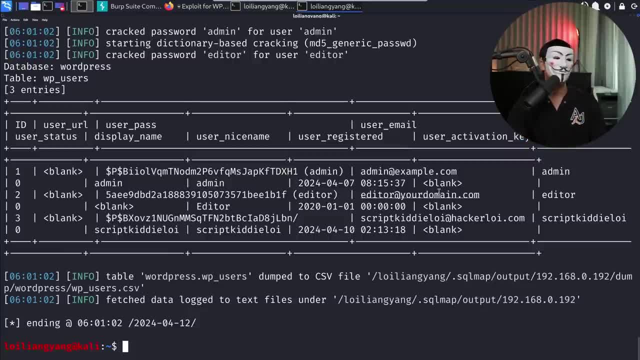 for this. let's see whether we can get any hit for that. and boom, you can see, right here we get a following, we got the user admin and we got its password of admin too. so, heading back to the site, I can go ahead and to slash WP dash login. 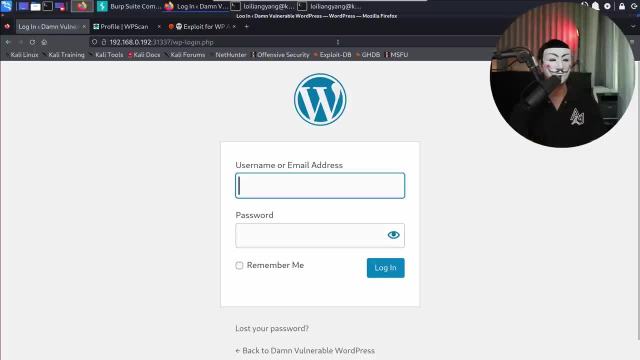 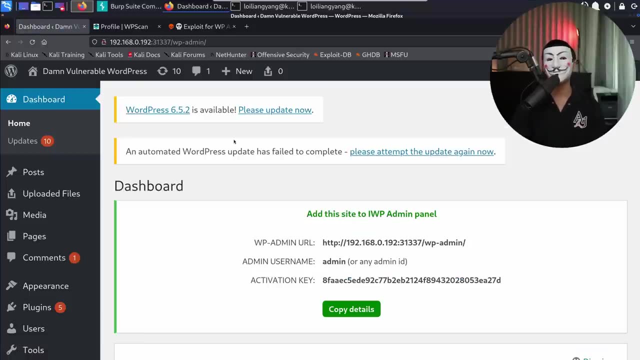 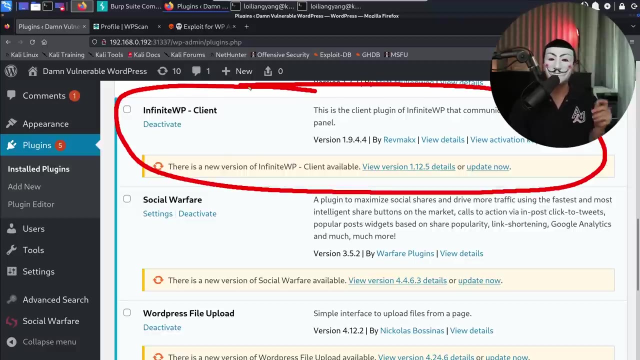 hit enter on this because this is the default login page for WordPress. enter admin, admin, click login and boom, we're in. we've gotten access into the site and heading over into the installed plugins you can see right here of infinite WP client, and this also has a significant critical vulnerability that we can. 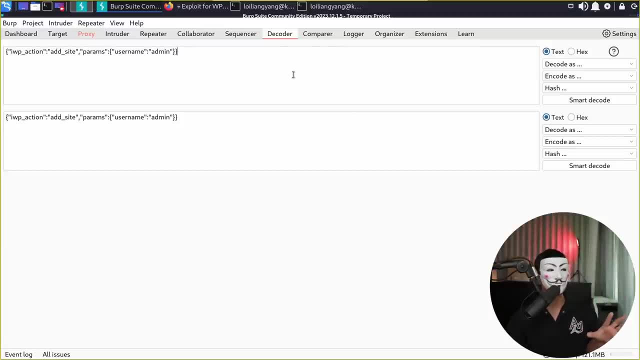 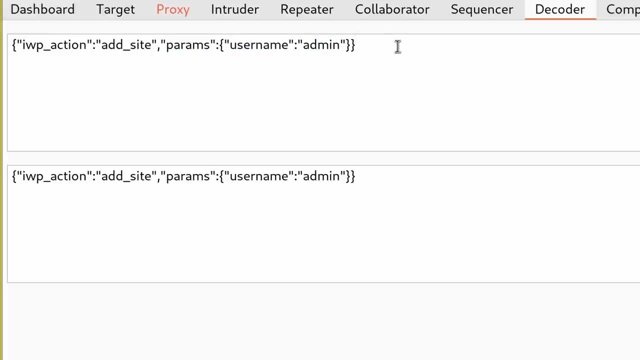 target and what's really cool right here, we have to payload that we can use. so we have the following of IWP action at site params, user admin. so what we can do here now is to go ahead and encode this into base 64, and we're going to use this. 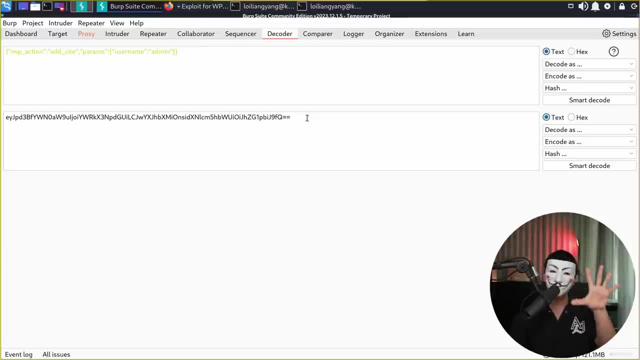 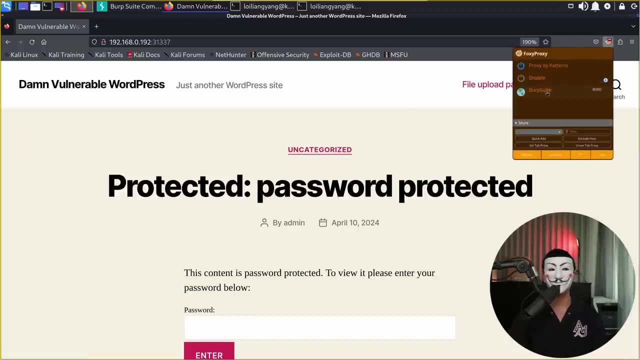 to send to a specific part of the site, allowing us to gain administrative access to the site. you can see right here I've locked out of the side and what I can do is again go to the top right corner. I click under say burp suite to be our interceptor. I click on to the site again. I go back to burp suite under. 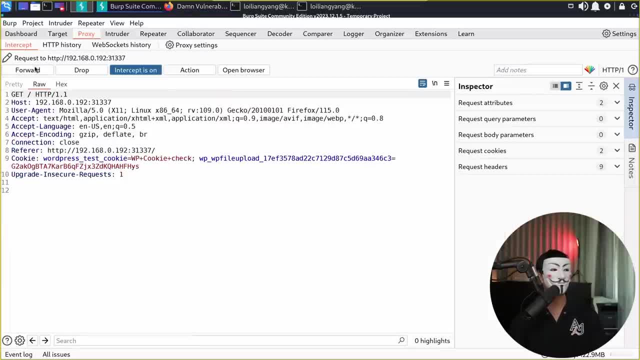 the proxy tab. what I can do now is go ahead and forward this and this may be the request. okay, let me just go ahead and click on it one more time. and now we have interception. so what i can do here now is to go ahead and target this with the specific exploit against the plugin. here right at the bottom. we